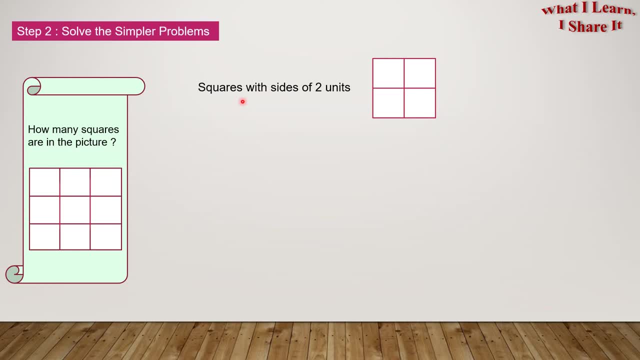 Now we'll be starting with squares with the sides of 2 units, which looks like this: And here is our model again: 1,, 2,, 3, and 4.. Number of two unit squares equals four. Now we'll be doing squares with sides of three units. 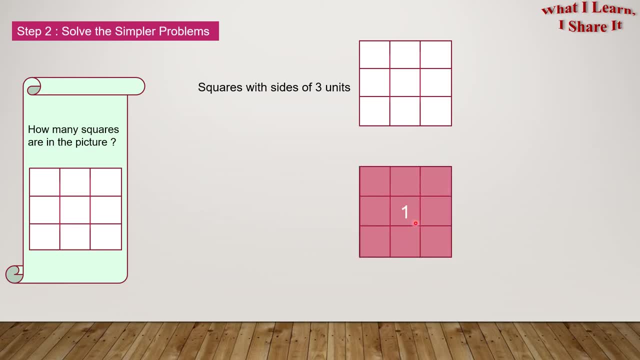 And here is our model. And there is one square with sides of three units. Number of three unit squares equals one. Step three: Use the answers to the simpler problems to solve the original problem. So how many squares are in the picture? Squares with sides of one unit equals nine. 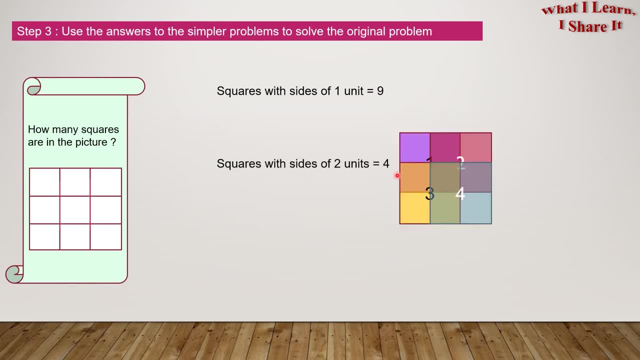 Squares with sides of two units equals four. Squares with sides of three units equals one. Number of squares in the picture equals nine plus four plus one equals fourteen. Yay, We solved the problem. Coming up is the fun part, and that is. 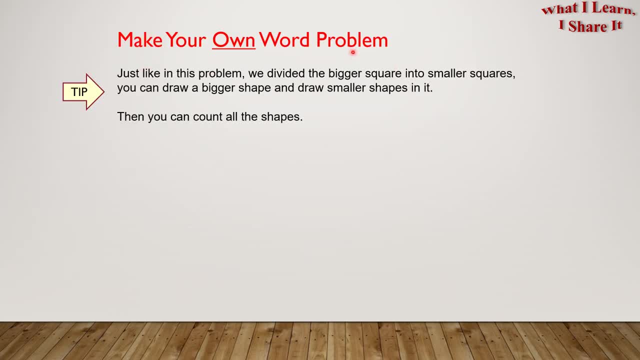 Make your own word problem. Here is a tip. Just like in this problem, we divided the bigger square into smaller squares. You can draw bigger shapes and draw smaller shapes in it. Then you can count all the shapes. Here is an example. 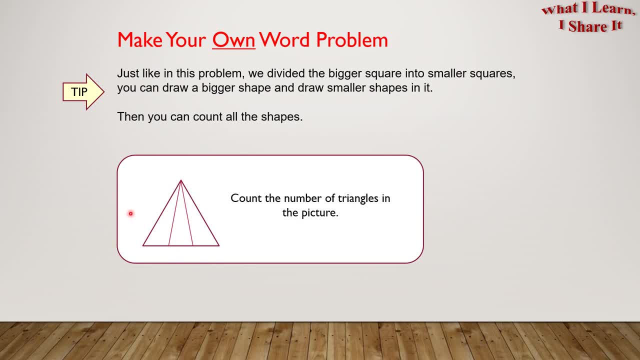 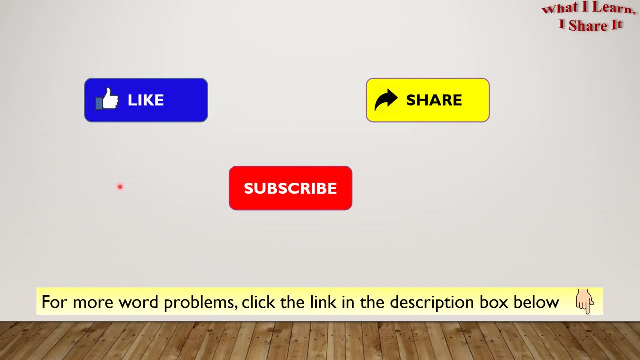 Count the number of triangles in this picture. So easy to make your own word problems. For more word problems, click the link in the description box below. Hope you like my video. Thanks for watching. Please like, share and subscribe to my channel. See you, Bye.